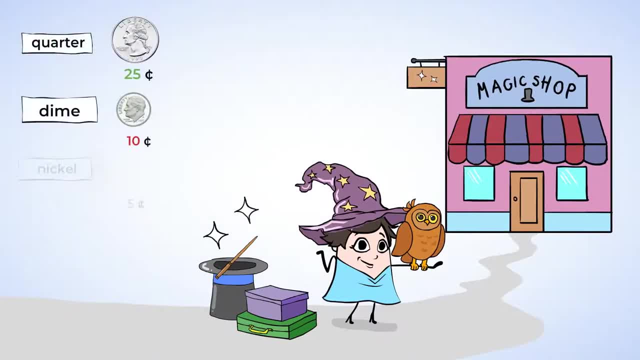 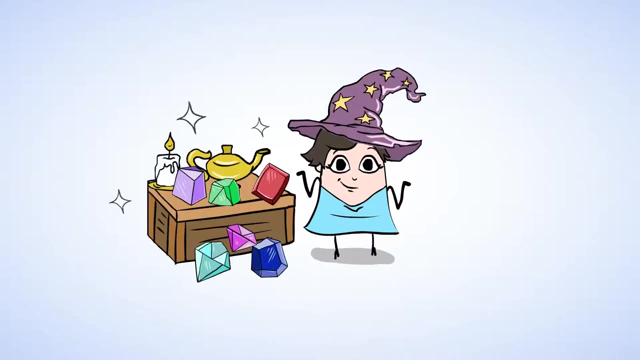 the video. We will be using quarters, dimes, nickels, pennies and dollar bills to practice today. If you want, you can pause this video now to go get some coins and dollar bills. Okay, now let's get started. These magic crystals are so sparkly. A mini pink one costs 43 cents. 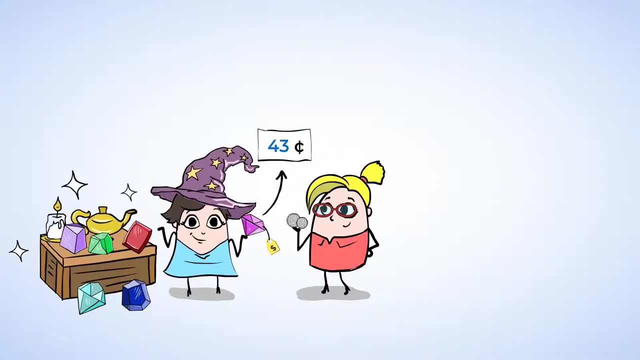 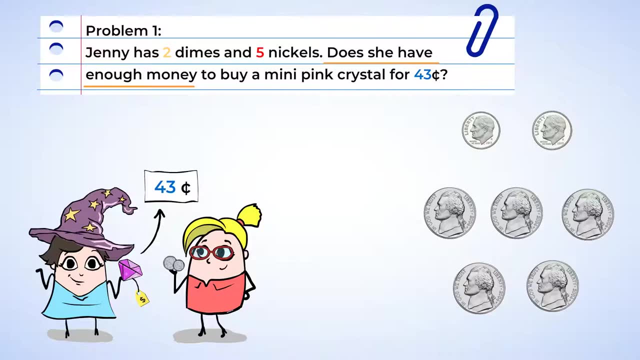 and a customer named Jenny comes in with some coins in her pocket. The coins are shown below. Does she have enough to buy a mini pink crystal? Jenny has two dimes and five nickels in her pocket. To figure out how much money she needs to buy a mini pink crystal, she has to buy a. 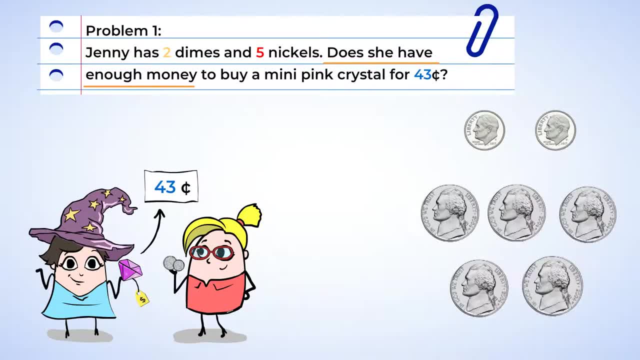 We can find the value of the dimes, the value of the nickels, and then add them together to get the total value. A dime is worth 10 cents, So two dimes are worth 20 cents because 10 plus 10. 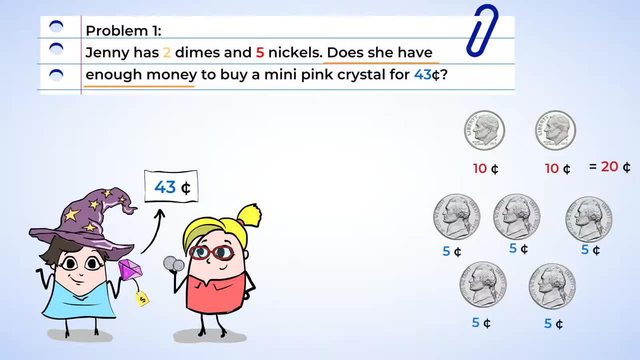 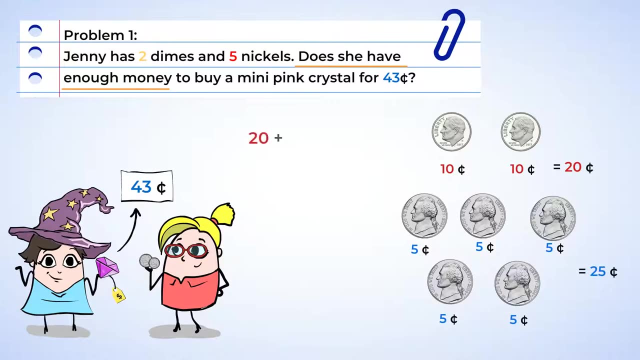 is 20.. A nickel is worth 5 cents. Jenny has five nickels, so you can skip count 5,, 10,, 15,, 20, 25.. Jenny has 25 cents in nickels. Now add 20 and 25.. 20 plus 25 is 45. Jenny has 45 cents, Since 45 is bigger than 43,. 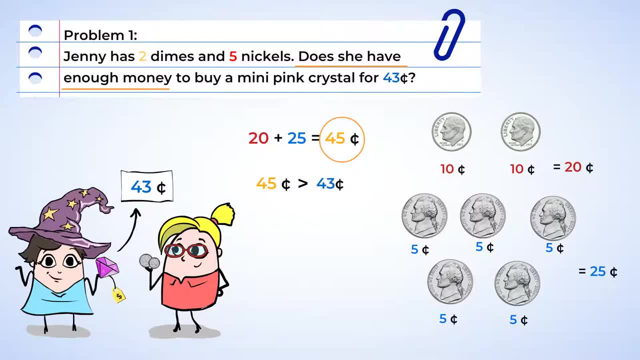 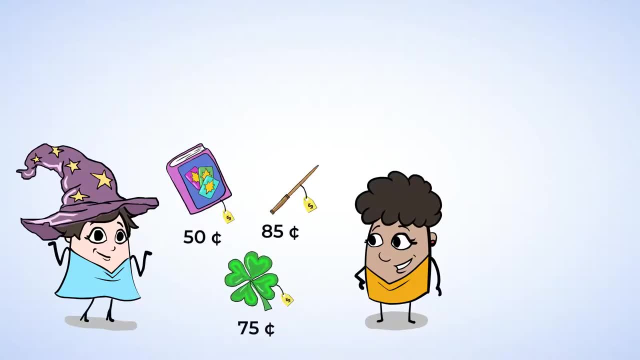 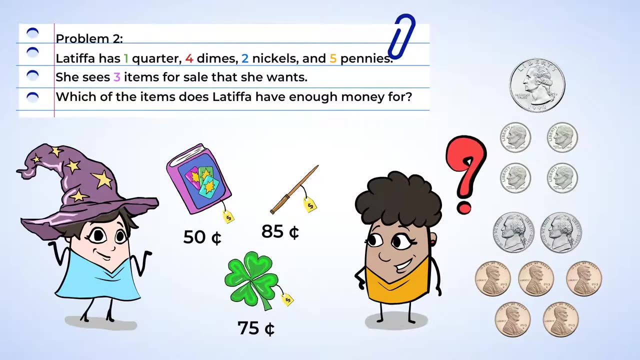 Jenny has enough money for a mini pink crystal- Nice. She'll be so happy to hear that Latifah comes in next, also with some coins in her pocket. Here are all the coins in Latifah's pocket. Latifah is still deciding what to buy. She might want a little book on card tricks. 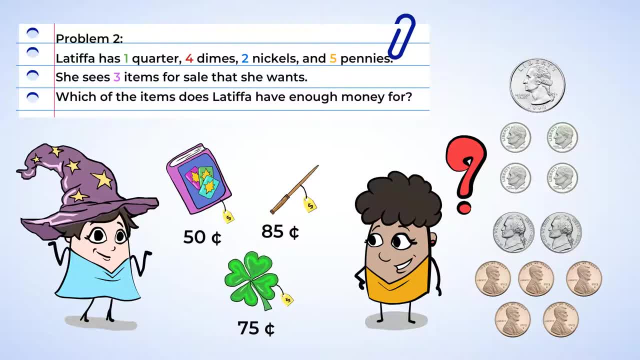 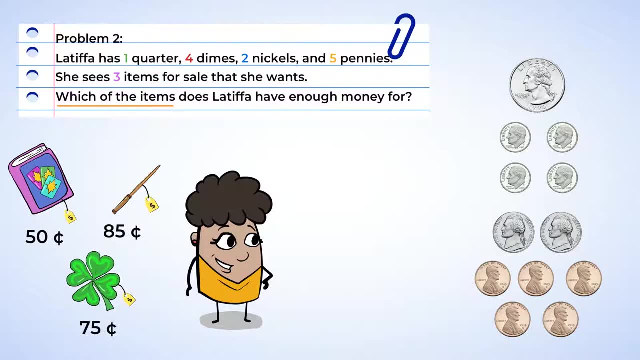 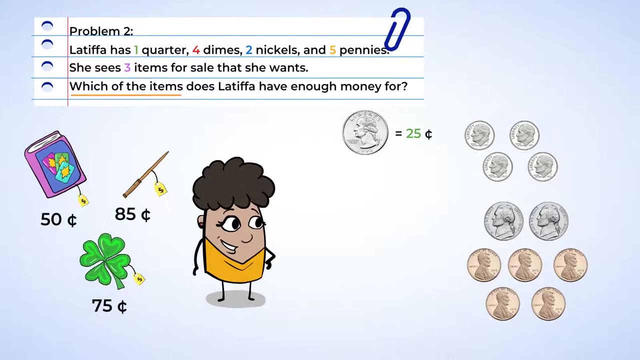 a new magic wand or a lucky four-leaf clover charm. We can check to see if she has enough money for these items. First, let's figure out how much money Latifah has with her. She has one quarter, which is worth 25 cents. She has four dimes. A dime is worth 10 cents, 10,, 20,, 30,. 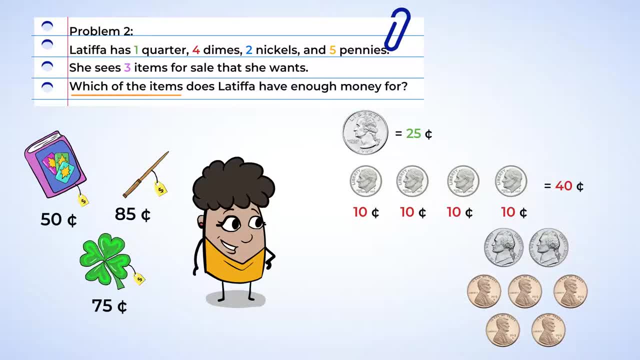 40. So she has 40 cents worth of dimes. Two nickels is worth 10 cents. 5 plus 5 is 10.. Lastly, a penny is worth 1 cent, so 5 pennies is 5 cents. Now we can add up the. 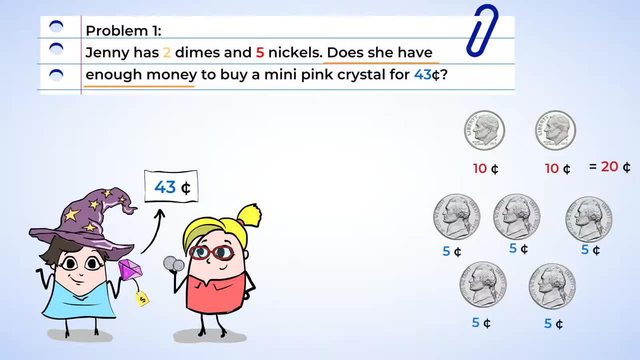 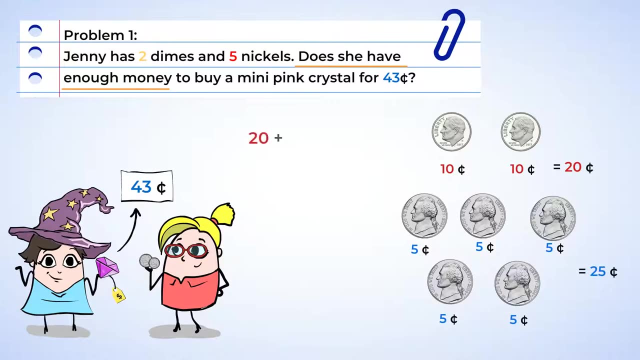 is 20.. A nickel is worth 5 cents. Jenny has five nickels, so you can skip count 5,, 10,, 15,, 20, 25.. Jenny has 25 cents in nickels. Now add 20 and 25.. 20 plus 25 is 45. Jenny has 45 cents, Since 45 is bigger than 43,. 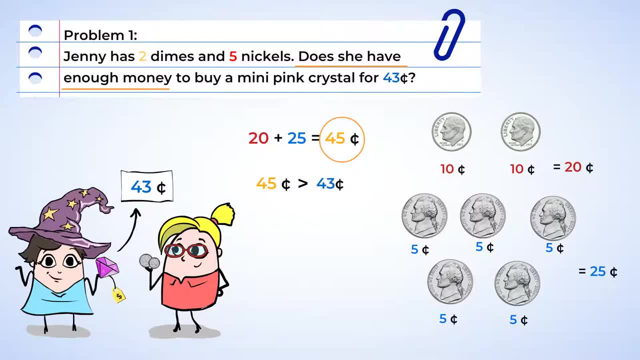 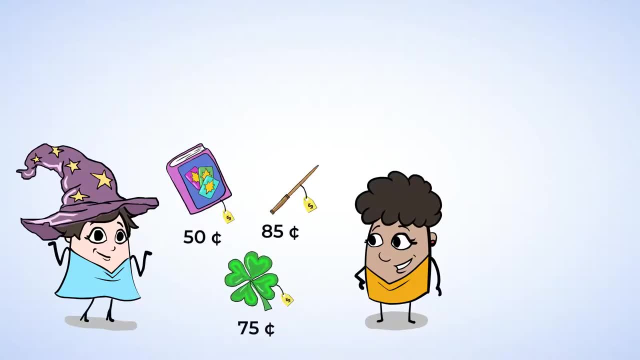 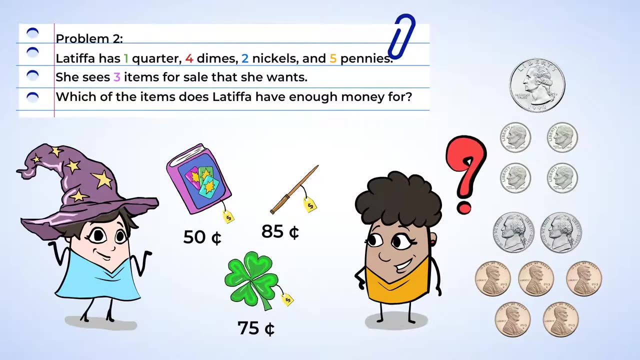 Jenny has enough money for a mini pink crystal- Nice. She'll be so happy to hear that Latifah comes in next, also with some coins in her pocket. Here are all the coins in Latifah's pocket. Latifah is still deciding what to buy. She might want a little book on card tricks. 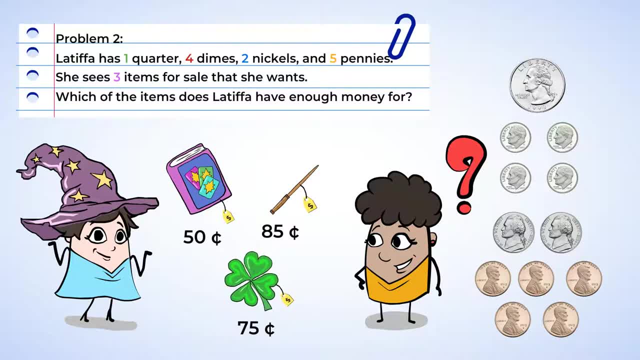 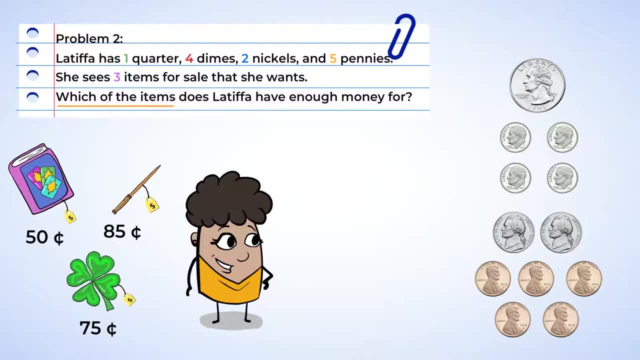 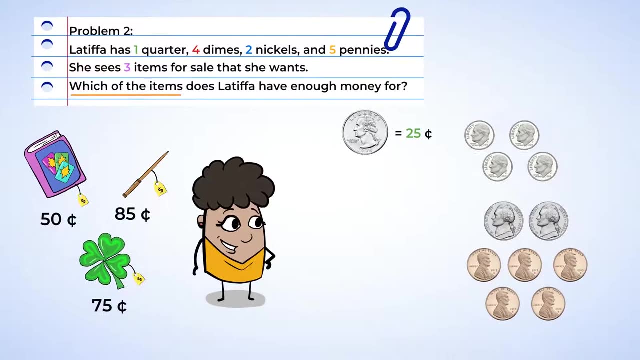 a new magic wand or a lucky four-leaf clover charm. We can check to see if she has enough money for these items. First, let's figure out how much money Latifah has with her. She has one quarter, which is worth 25 cents. She has four dimes. A dime is worth 10 cents, 10,, 20,, 30,. 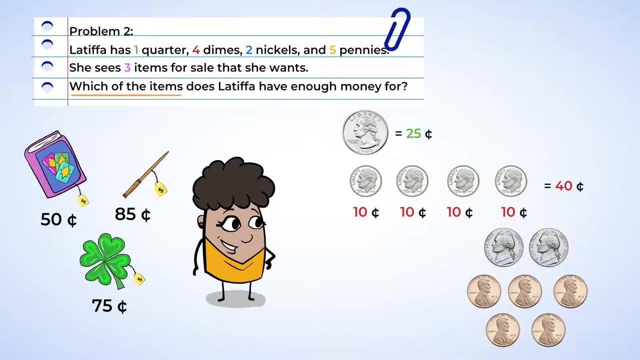 40. So she has 40 cents worth of dimes. Two nickels is worth 10 cents. 5 plus 5 is 10.. Lastly, a penny is worth 1 cent, so 5 pennies is 5 cents. Now we can add up the. 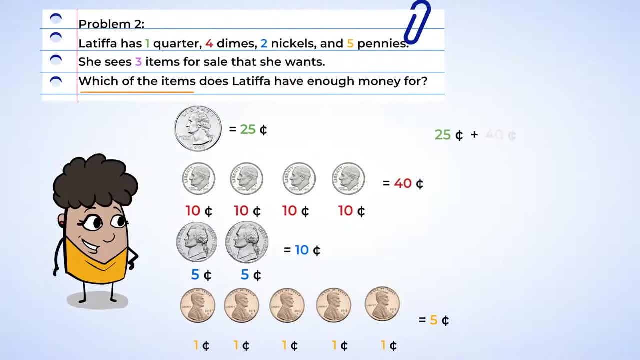 values to find the total amount. 25 and 40 is 65.. You can skip count by 10s, starting from 25, to figure this out. Next, 65 plus 10 more is 75.. Lastly, 75 plus 5 is 80.. So Latifah has 80 cents. 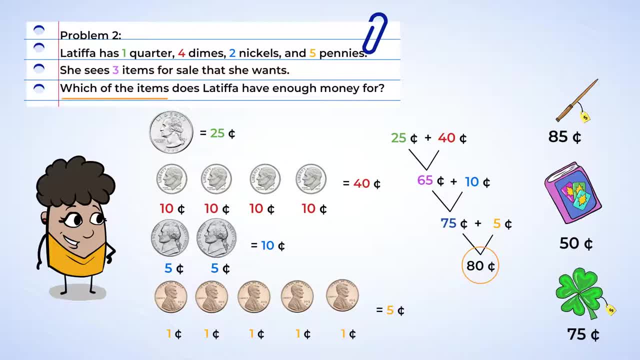 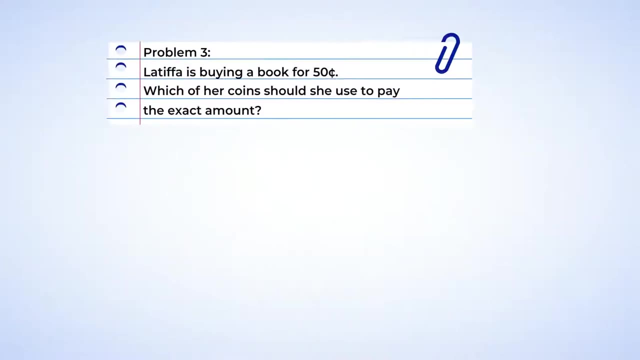 Look at the items to find the ones that are 80 cents or less, to find what Latifah can buy. The magic wand is 85 cents, so she cannot buy that, But the book is 50 cents and the charm is 75 cents, so Latifah can buy either of those. Thanks for helping Latifah out. It looks like. 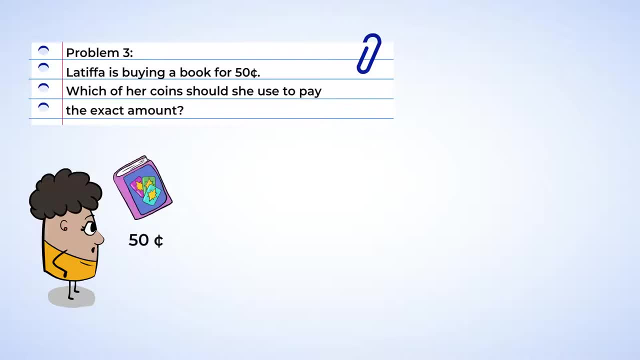 Latifah has decided to buy the book on card tricks. That sounds like fun. Which coins should Latifah give the cashier to exactly pay for the book? We need to decide which of Latifah's coins to use. that will add up to exactly 50 cents. 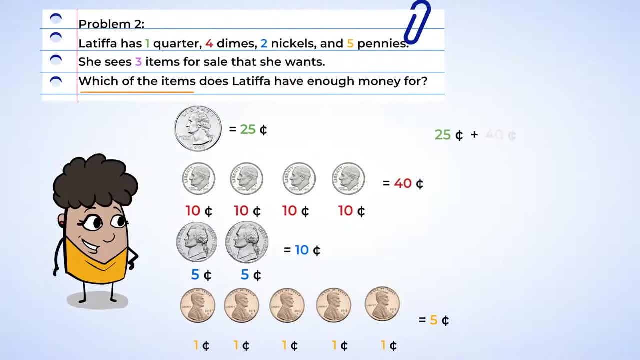 values to find the total amount. 25 and 40 is 65.. You can skip count by 10s, starting from 25, to figure this out. Next, 65 plus 10 more is 75.. Lastly, 75 plus 5 is 80.. So Latifah has 80 cents. 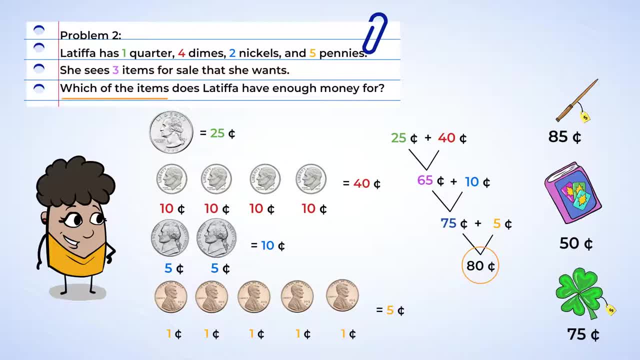 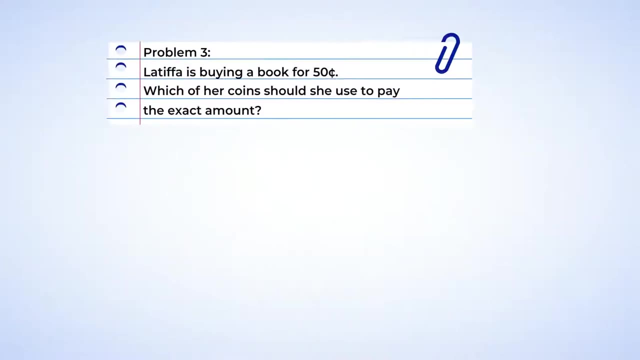 Look at the items to find the ones that are 80 cents or less, to find what Latifah can buy. The magic wand is 85 cents, so she cannot buy that, But the book is 50 cents and the charm is 75 cents, so Latifah can buy either of those. Thanks for helping Latifah out. It looks like. 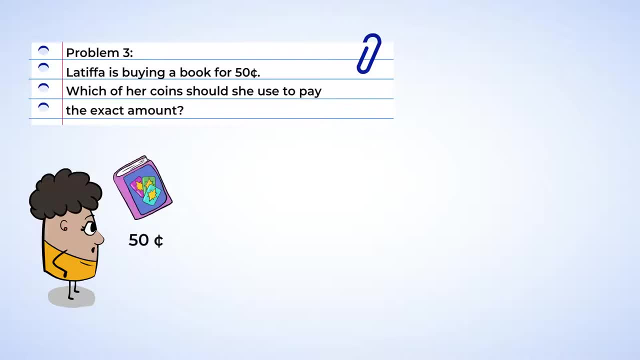 Latifah has decided to buy the book on card tricks. That sounds like fun. Which coins should Latifah give the cashier to exactly pay for the book? We need to decide which of Latifah's coins to use. that will add up to exactly 50 cents. 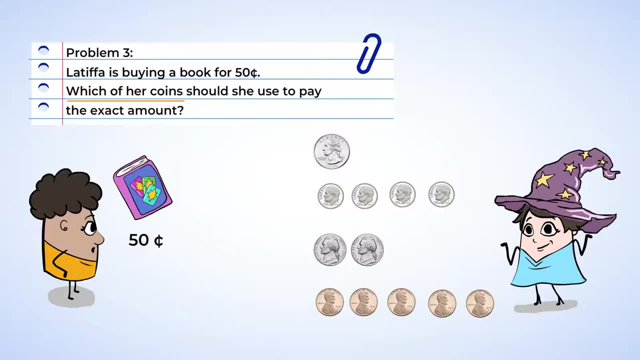 When figuring this out, two things are very helpful to remember. First, always start with the coin that has the largest value, in this case the quarter. Next skip counting will be your friend. So start with the quarter- 25 cents. Next use the dimes and skip count by 10s. But 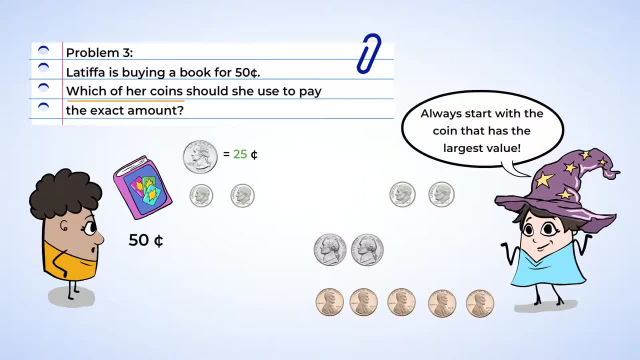 don't go over 50 cents: 25,, 35,, 45.. The next dime would make 55 cents, so we can't use any more dimes. Now on to nickels. Skip count by 5s, starting at 45,, but don't go over 50. 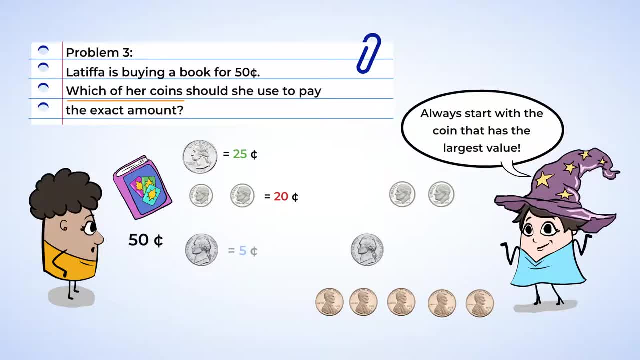 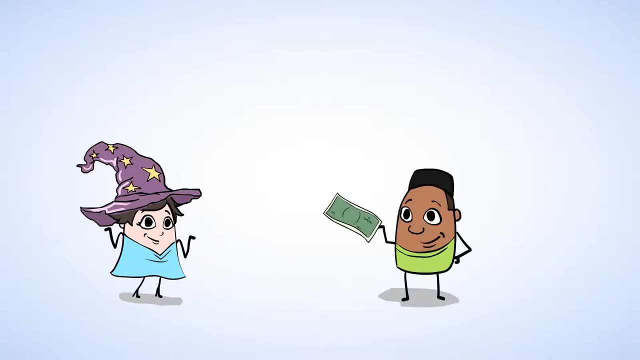 45, 50.. That's it, We're done. We have reached 50 cents exactly and we used 1 quarter, 2 dimes and 1 nickel. Great job. It looks like another customer, Will, has come into the store. He has a $1 bill that he can spend. 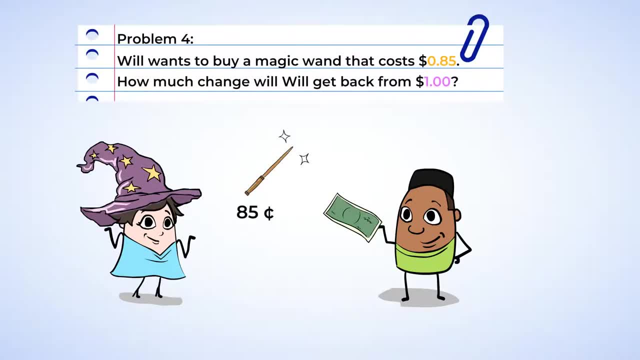 and he wants to buy that magic wand that costs 85 cents. When Will gives the cashier the $1 bill, the cashier will give Will change When talking about money. change is what you get back when you pay more money than what something costs. So how much change will the cashier give Will? 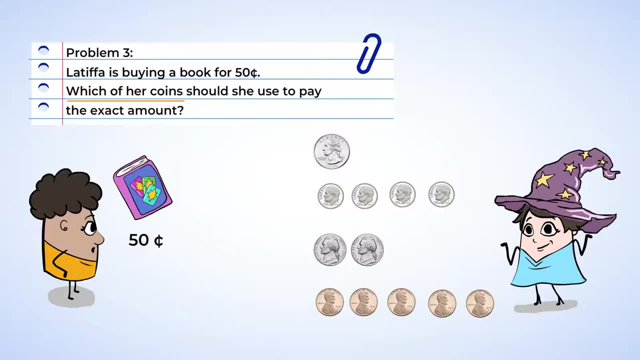 When figuring this out, two things are very helpful to remember. First, always start with the coin that has the largest value, In this case the quarter. Next skip counting will be your friend. So start with the quarter- 25 cents. Next use the dimes and skip count by 10s. But 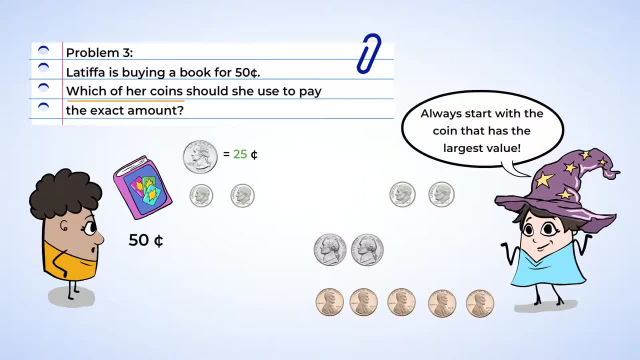 don't go over 50 cents: 25,, 35,, 45.. The next dime would make 55 cents, so we can't use any more dimes. Now on to nickels. Skip count by 5s, starting at 45,, but don't go over 50. 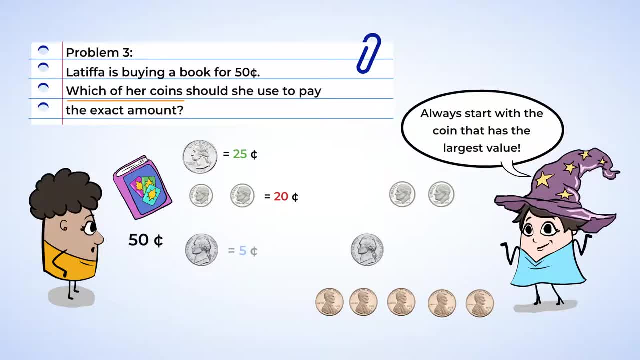 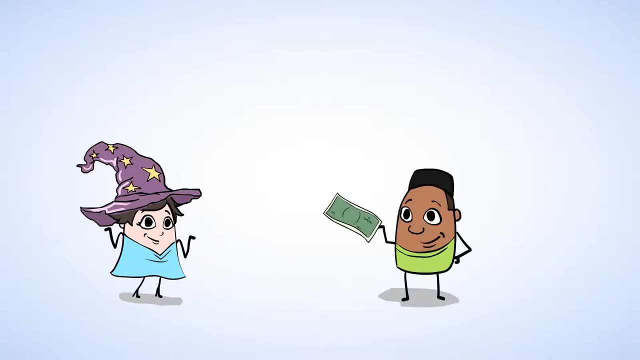 45, 50.. That's it, We're done. We have reached 50 cents exactly and we used 1 quarter, 2 dimes and 1 nickel. Great job. It looks like another customer, Will, has come into the store. He has a $1 bill that he can spend. 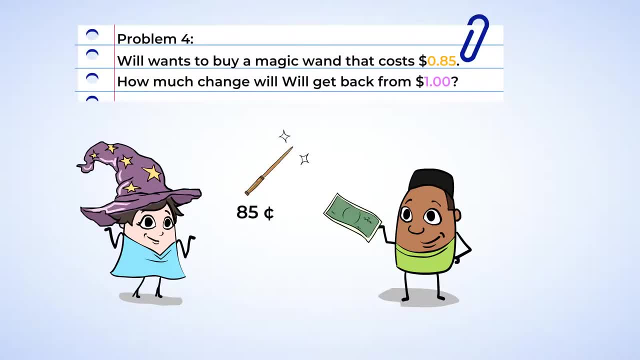 and he wants to buy that magic wand that costs 85 cents. When Will gives the cashier the $1 bill, the cashier will give Will change When talking about money. change is what you get back when you pay more money than what something costs. 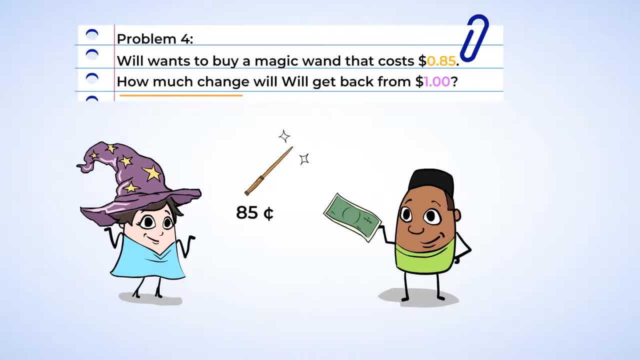 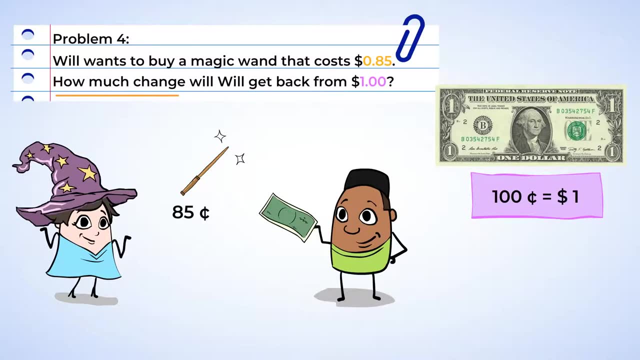 So how much change will the cashier give Will? First, we need to remember that $1 is the same as 100 cents, So Will has 100 cents and the magic wand costs 85 cents. We need to subtract the 85 cents from: 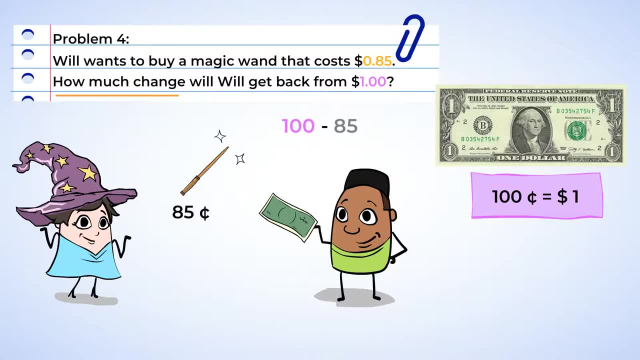 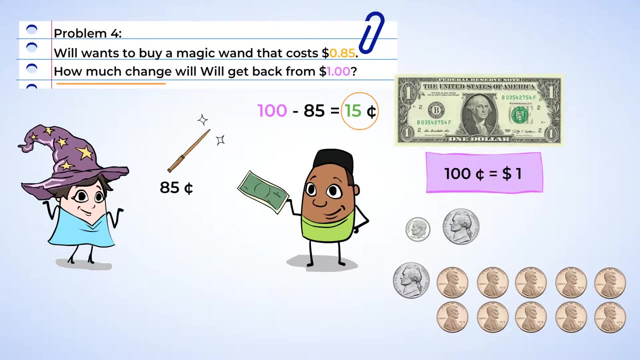 the 100 cents. 100 minus 85 is 15.. So Will will get 15 cents in change. Which coins do you think he will get? Maybe 1 dime and 1 nickel, Or possibly a nickel and 10 pennies. What other? 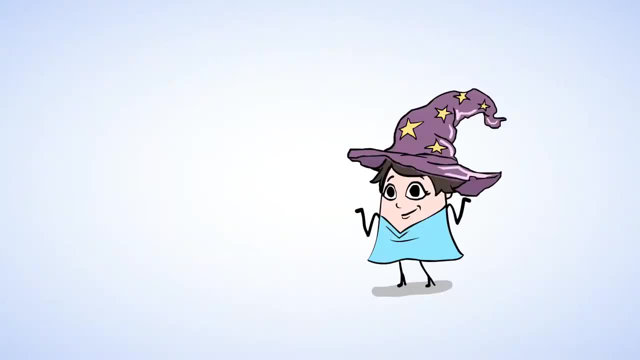 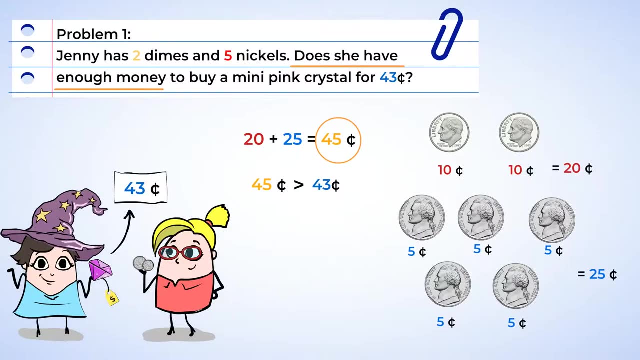 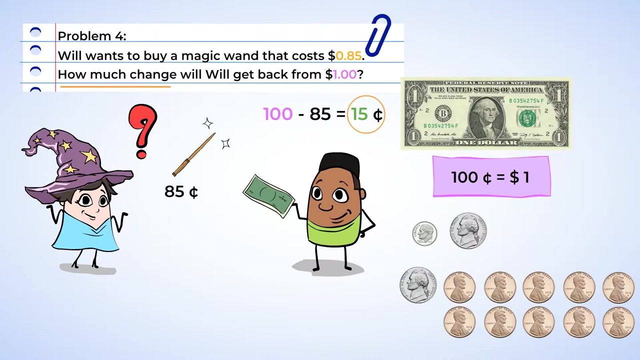 options. can you think of Great work today? You worked on all sorts of money word problems. You added up the value of coins to figure out if there was enough money to buy an item. You also learned about change and that you need to subtract to find the amount of change that you will get. Like any word problem, you always can. 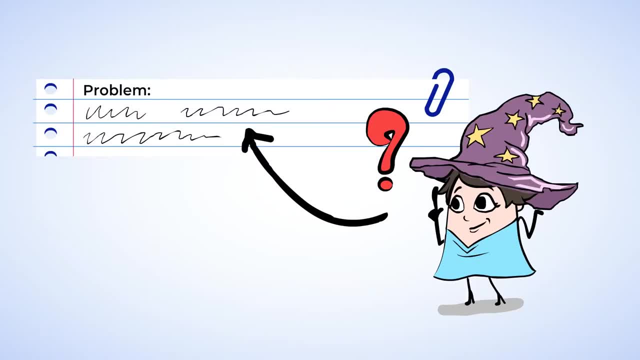 look for clues by asking yourself what is happening in the problem. See you soon.